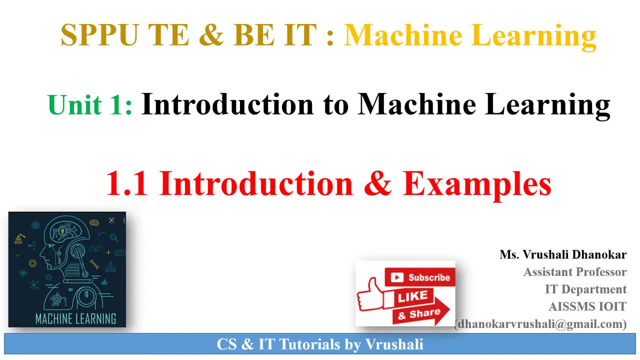 Okay, so the subject name is machine learning for T and the subject name is machine learning and application for B. So this session will start from the first unit and the unit name is introduction to machine learning, And in this session we will learn the first point: introduction and example. 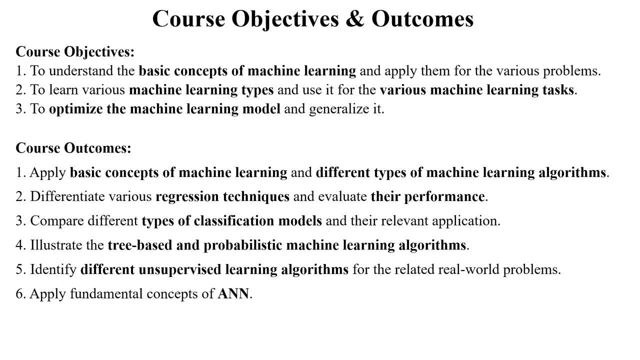 So, before start the session, the important thing, why this subject included in your syllabus. So there are some course objectives and course outcomes. See here. the course objective is, you know, you should understand some basic concepts of machine learning, to apply various problems and also to learn various machine learning types and various machine learning tasks. 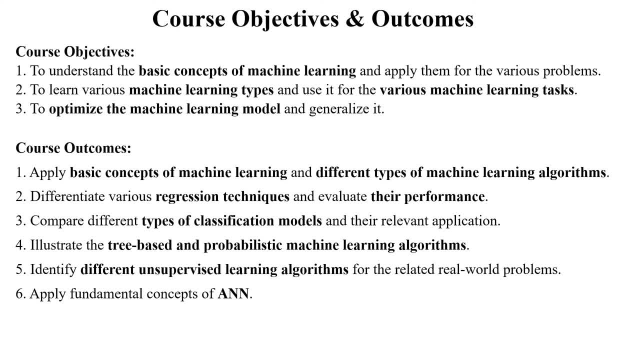 And again, another objective of machine learning is to optimize the machine learning model and also generalize it. Now the next one is outcome. What is the outcome of machine learning subject? The outcome of machine learning subject is: you should apply basic concepts of machine learning. 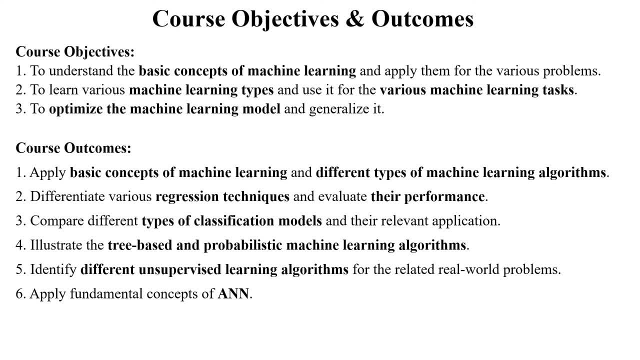 And by applying different types of machine learning algorithms you should understand, differentiate various regression techniques than their performances. Again, compare different types of classification models, Then also their relevant application than some tree based, and probability machine learning algorithms, than some unsupervised learning algorithms. 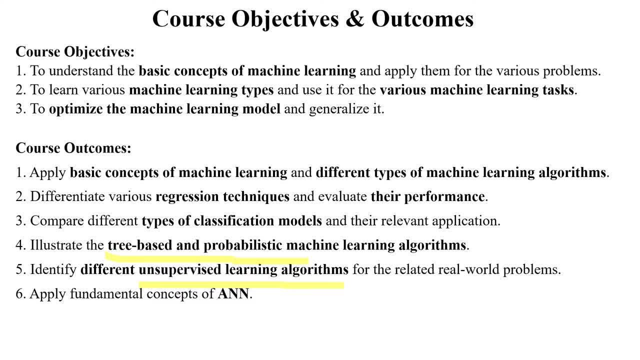 Okay, and we will also learn these all techniques by using some real world problems, And we also learn about some fundamental concepts- Okay, And we will also learn about some fundamental concepts of ANN. So this is, just course, objective and outcome of machine learning. subject: 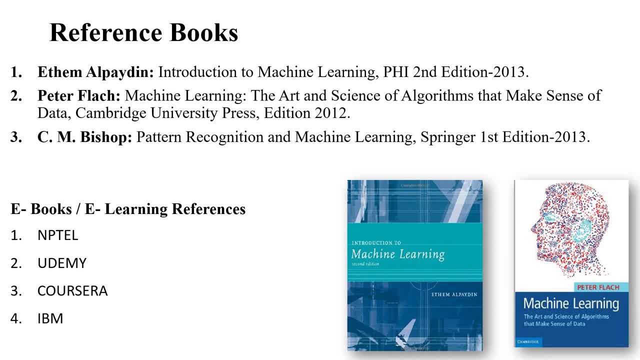 Next. Now, next thing is reference books. So there are item applied in this author reference book that is introduction to machine learning. The PDF is also available on the net. Okay, This is one of the most useful book for machine learning purpose. 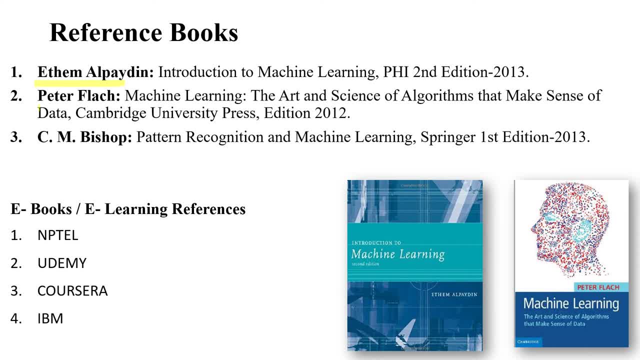 Again. the another book is Peter Fage. Okay, Peter Fage, This is one of the most useful book for machine learning- the art and science algorithm. and the another book is CM Bishop- pattern recognition and machine learning. So you should refer this reference books for study purpose, and PDF is also available on the net. 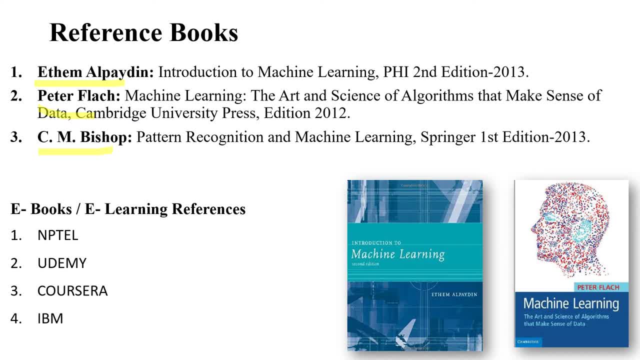 Now there are some ebooks and e-learning references, So we know that there are lots of videos are available on the YouTube regarding machine learning subjects. So you should complete NPTEL, Udemy, Then Coursera, IBM, this kind of courses. 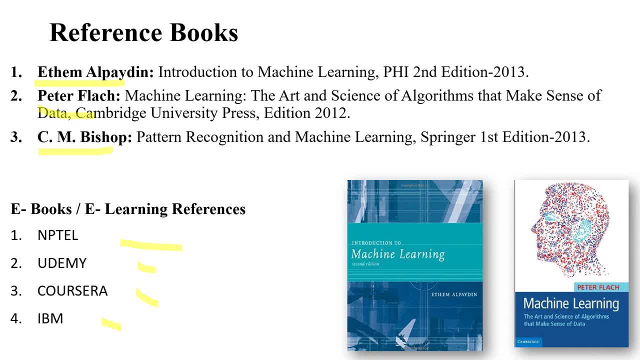 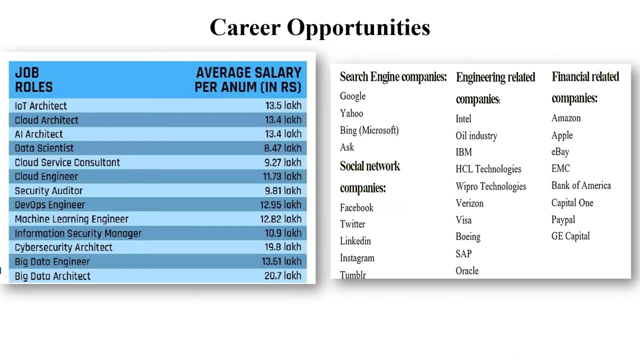 So this kind of best course for the machine learning. So you should complete those courses and you should refer those courses and books Next. Now, the next thing is: what are the career opportunities of machine learning? So we know that the machine learning is a recent trends, or career trends nowadays. 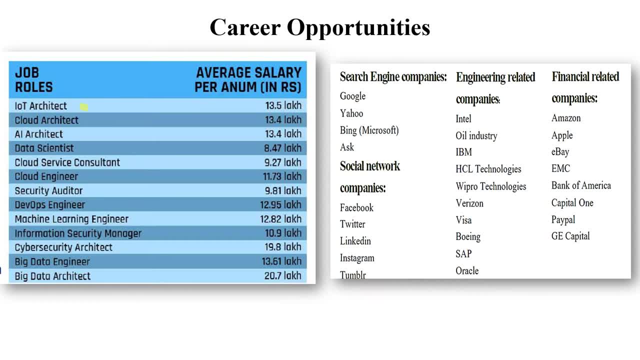 Now there are various job roles like IOT architect, Then cloud architect, AI architect, data scientist. Then again there are positions like cloud service consultant, cloud engineer, then a security auditor, devops engineer, machine learning engineer, then information security manager, cyber security architect, big data engineer and big data architect. 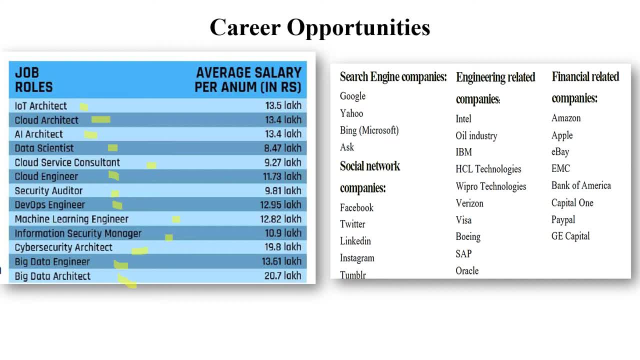 So these are the job roles provided by the machine learning concepts and machine learning individuals. Okay, Now, these are the some companies like there are various service based products. There are various service based product based companies. They also offer machine learning engineers. Like, again, there are some companies like Google, Yahoo, then Facebook, Twitter, LinkedIn, Instagram. 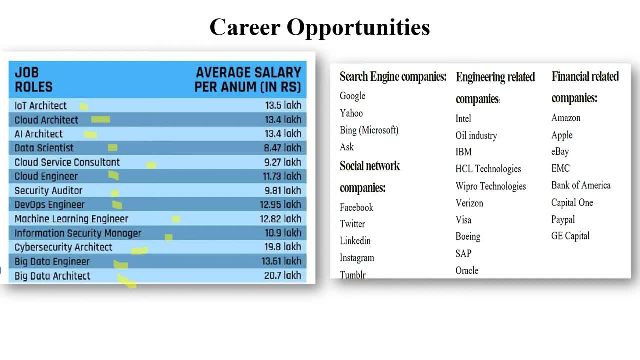 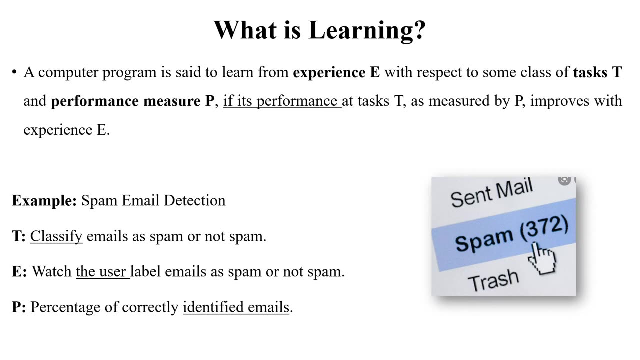 Nowadays each and every field: machine learning, then data science, this kind of concepts generally used. Okay, So these are the just career opportunity and this is recent trends nowadays Now. so let's start the unit wise point Now, before start: what is mean by machine learning? 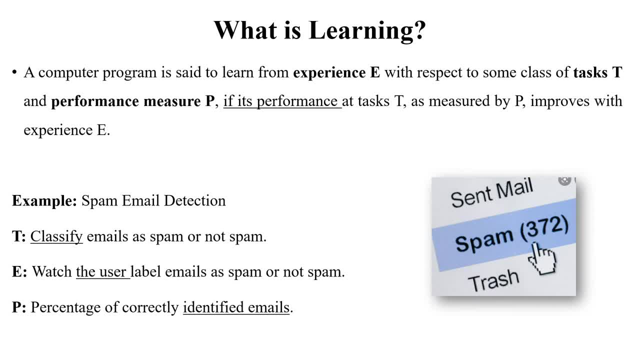 The first thing is what is mean by learning. So learning basically has three components, that is, experience, which declared as a E, then task, which declare as a T, and performance major, which declare as a P. So E, T and P, these are the three main components of learning. 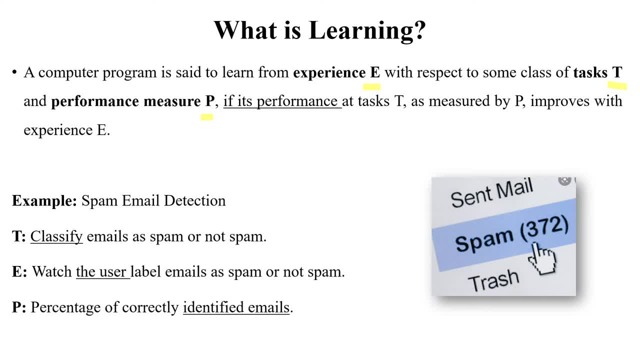 Now let's see what is meaning of that. So let's take one example. The example is spam email detection. Okay, So we need to classify those things into the three parts, that is, experience, task and performance. Now you know that spam emails- spam emails- is the unwanted emails. 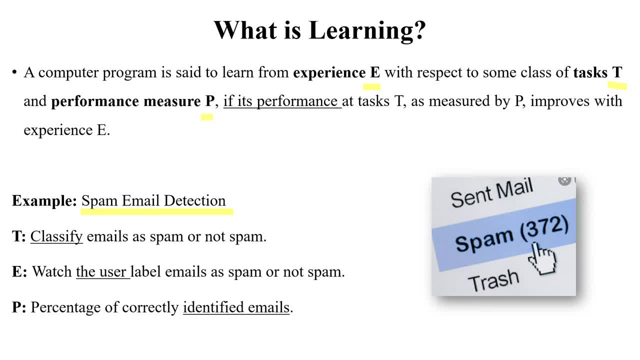 Okay, Like there are different emails related to the offers, related to the discounts, right, This all emails are goes to the spam folder, So you need to classify those emails. The particular email is spam email or not a spam email. Okay, So this is your task. 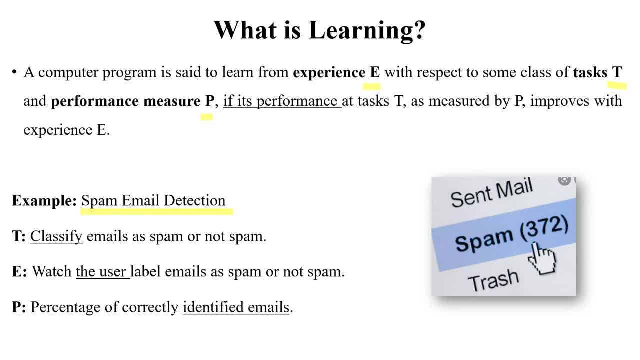 The first component is task and the task is classify email, whether the particular email is spam or not spam. Okay, So first task is classify. The next is experience. Experience means what user find out regarding this spam emails. User find out the particular level of that particular email is spam and level of that particular email which is not spam. 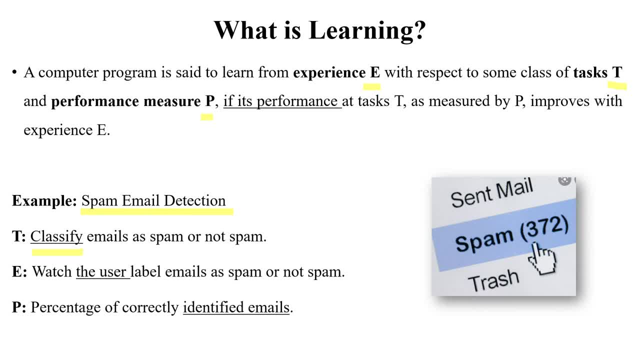 Generally not spam, Usually stored into this inbox and updates folder, Right. So user experience, those thing, User experience that the spam emails goes to spam folder. So this is called as experience regarding to the user. And last one is a performance. So how we can measure the performance. 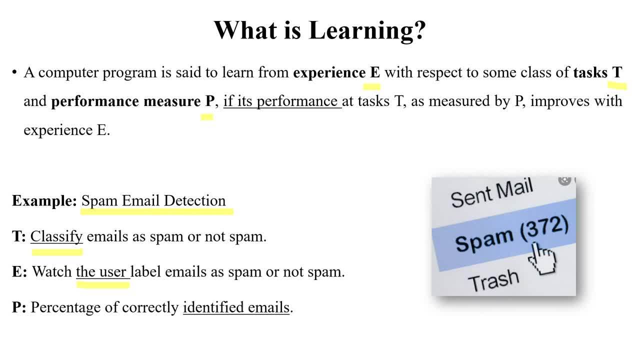 We can suppose measure the performance by using percentage means how many emails are correctly identified by the particular system, Right? So this is called as percentage. So this three things are called as learning means you should learn a particular system. So classify experience and a performance. that is, experience, task and performance. 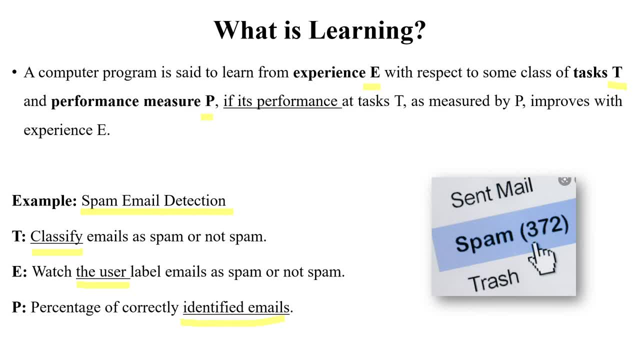 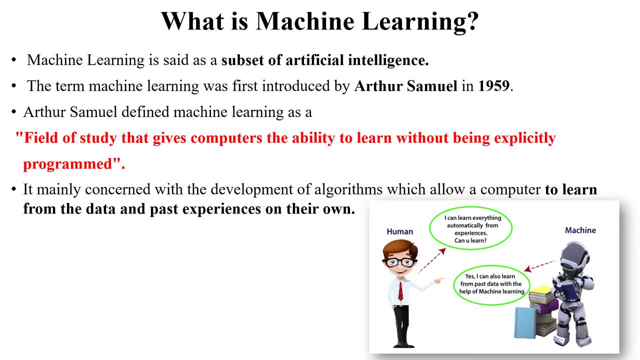 These three things are called as learning. Next. Now, the next and important thing is what is meant by machine learning. So we know that machine learning is just a subset of artificial intelligence. Okay, And deep learning is subset of machine learning. I will explain this thing on my next slide. 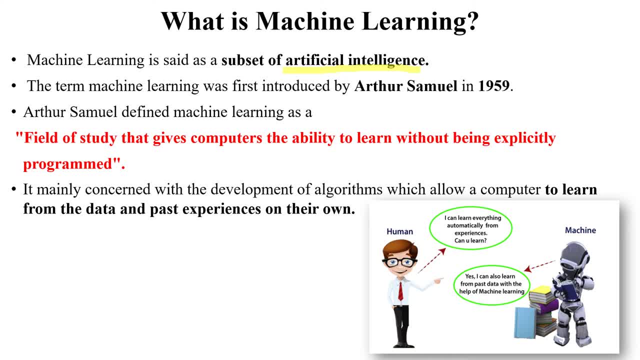 Okay, So the term machine learning was first introduced by author Samuel in 1959. And there are various definitions of machine learning. So what is basically what is meant by machine learning? See in your life user, learn from their past experiences, Right. 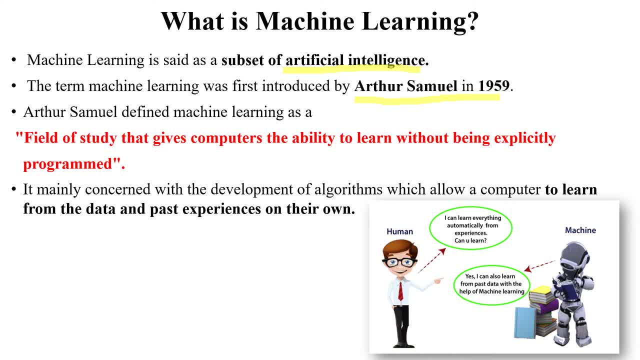 The particular human can be learned from their past experiences, or, as per their past experiences, they take a decision Right. So same thing happen with the machine Machine also can be learned from their past history or past search history, And as per their history, they take a particular decision. 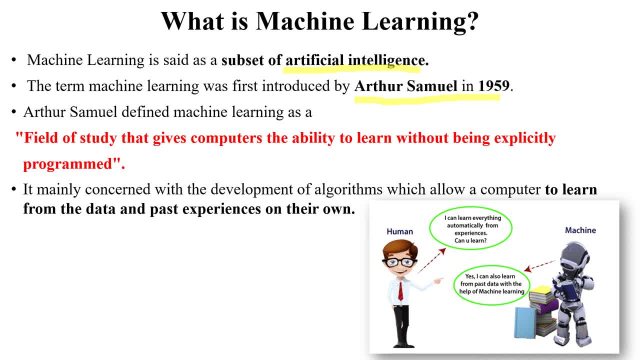 So this is called as machine learning. So this is just a definition, that is, field of study that gives a computer to ability to learn without being explicit To learn without being explicitly program. Okay, So machine can be learned by their past history, by their past experiences. 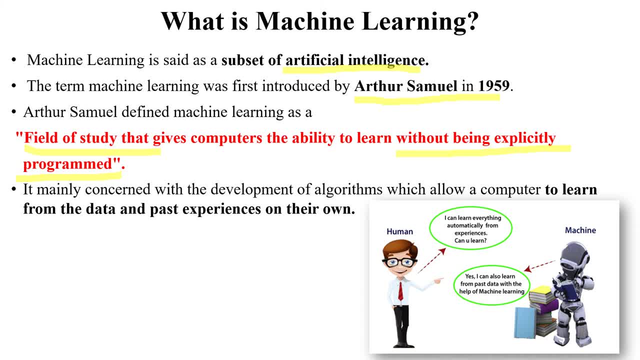 Okay, And as per their past experiences, they can predict the particular result or they can generate a data. So this is a concept of machine learning. So it may concern with the development of algorithms which allow computer to learn from data and past experiences on their own. 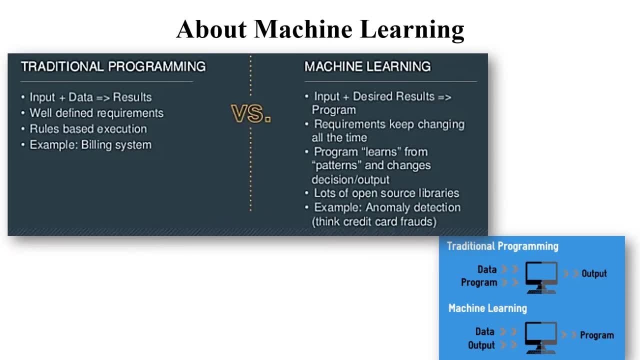 Okay, Next. Now see here again- This is in detail- concepts of machine learning. Now see here, there is one traditional programming and another with machine learning, Right, So we know that traditional programming, traditional programming means simply a C, C++ or Java, this kind of operations. 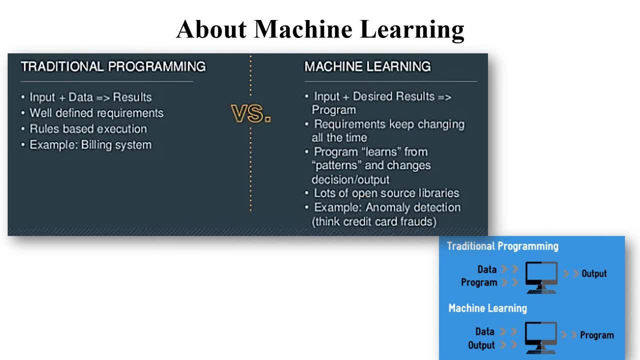 We will provide a particular input and the machine generated output Right. For example, arithmetic operation, We have provided 2 plus 2. Then machine generate the result. 4. In this traditional programming We use different loops, different for loops which cases, and different kinds of logics. 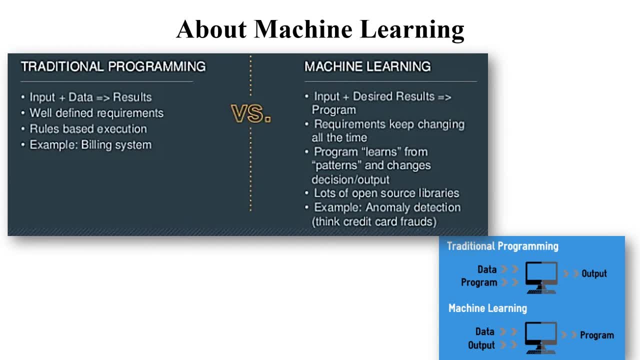 Right, For example billing system. But in machine learning? in machine learning we used data or different data sets for examining purpose. For example, suppose you should search different products on the Amazon or Flipkart. For example, you should search mobile on the Flipkart. 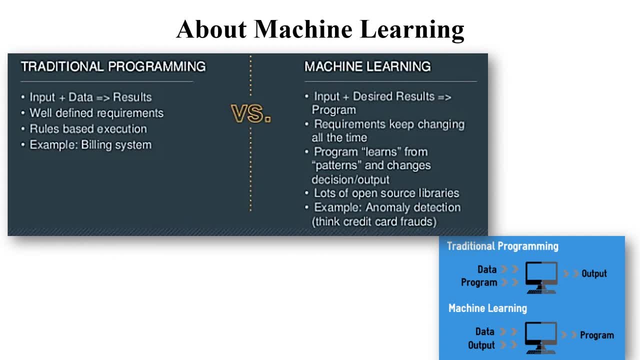 Okay, So next time when you open the particular Flipkart or Amazon application, It gives you a suggestion regarding this. Okay Means machine learn your history. machine learn that you should search a mobile on Flipkart or Amazon. Okay, So machine learn you from your search history and it shows you a suggestion like this: 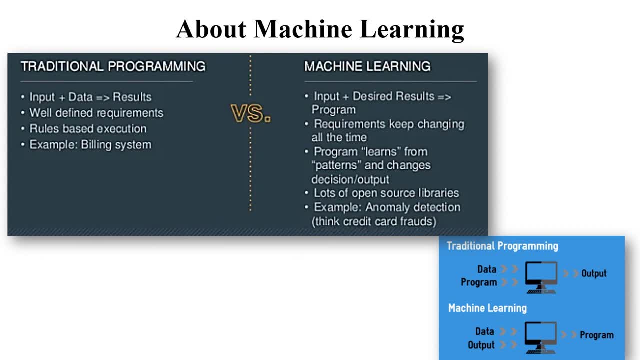 So this is called as machine learning. in machine learning, We will provide the particular data as the input and also desired result, So machine shows the suggestions regarding this. So the requirement of each and every users are different Requirements that will be keep changing all the time. 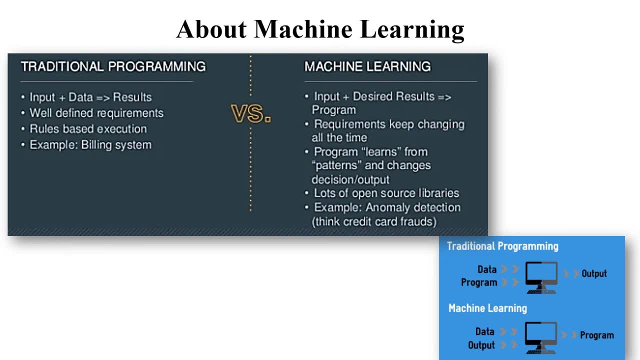 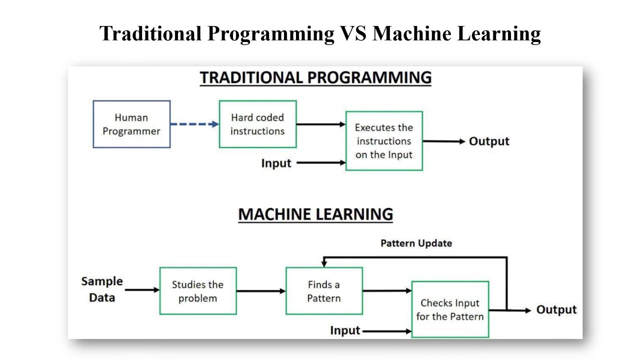 Right. So machine learn from the pattern, machine learn from the features and machine learn from the search history of the particular users. So this is called as machine learning. Now, this is just diagrammatical representation of traditional programming and machine learning in traditional programming. human programmer. 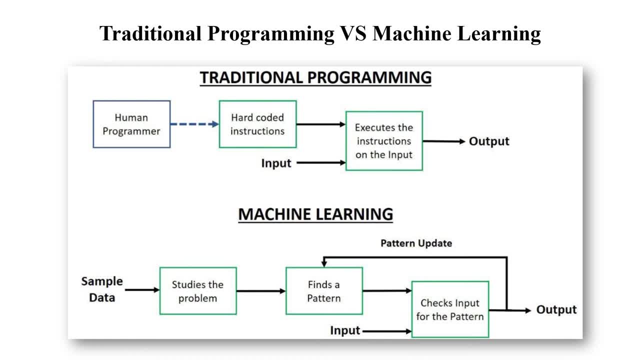 There is a hard-coded instructions, For example C, C++, Java, this kind of programming- Okay, And we execute those instruction on the input. Okay, For example arithmetic operations, and the particular result will be generated, that is, 2 plus 2 equal to 4.. 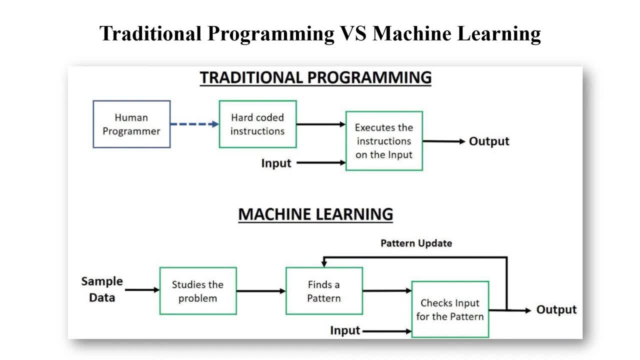 But in machine learning we will provide the sample data. For example, we will search mobile on the Flipkart. Okay, So machine study those problems. machines find out the pattern regarding your searches and they shows you some suggestions and some related things. related items as per your suggestions. 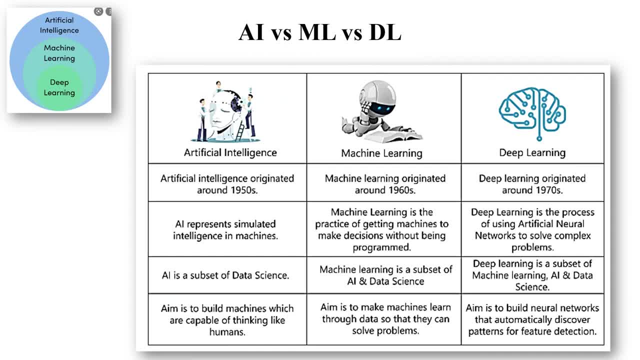 Right, So this is called as machine learning. Now, this is just difference between artificial intelligence, machine learning and deep learning. artificial intelligence generally originated in 1950, machine learning in 1960 and deep learning in 1970. So artificial intelligence- that is subset of data science and machine learning is a subset of artificial intelligence and deep learning is subset of machine learning. 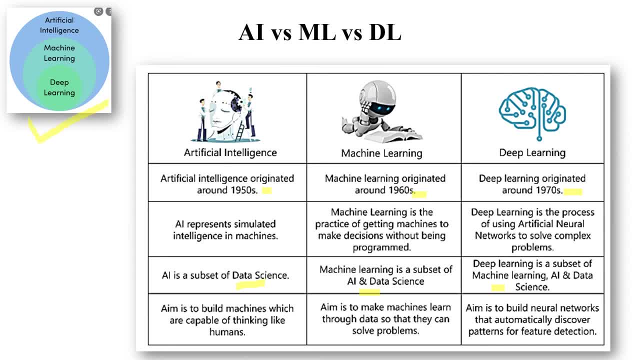 So this is just structure and representation of those things. So see, deep learning means deep learning build a neural network, Okay, Which work like a human brain and they learn the feature detection technique and features of each and every images. and machine learning generally used to learn from data and they use those data for solve a particular problem or predict the result, and the combination of machine learning and deep learning is called as artificial intelligence. 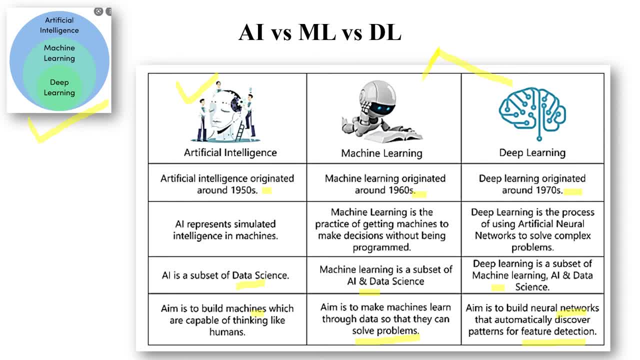 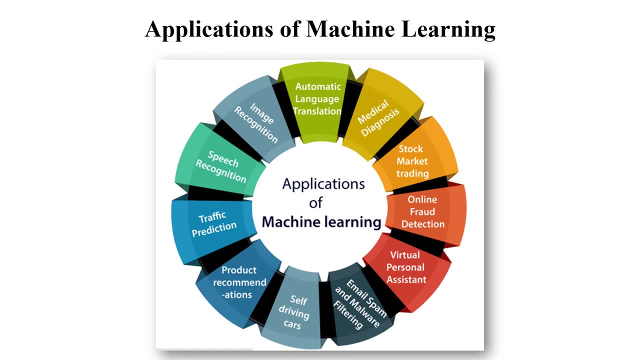 Artificial intelligence build a machine which is capable for thinking like a human. for that purpose, They use machine learning and deep learning, this kind of concept. Okay, So this is just difference between this. Now, these are the some applications of machine learning. nowadays, each and every field machine learning concept is used. that is medical diagnosis, stock market, online fraud detection, then virtual personal assistant, self driving cards, email detection, speech recognition, image recognition.